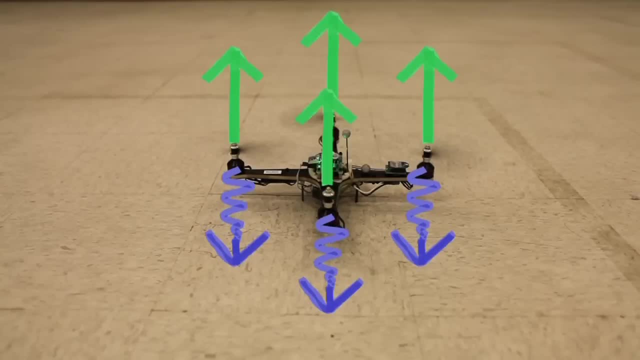 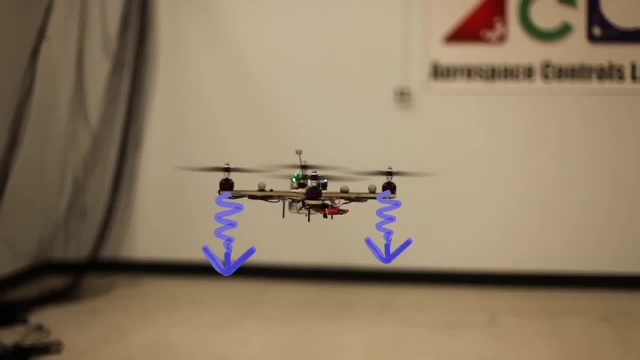 them. Newton's third law tells us that the air applies an equal and opposite reaction force on the propeller. When this lifting force equals that of gravity, the quadrotor has hover flight In order to bank, one propeller spins slightly faster than the opposite one. 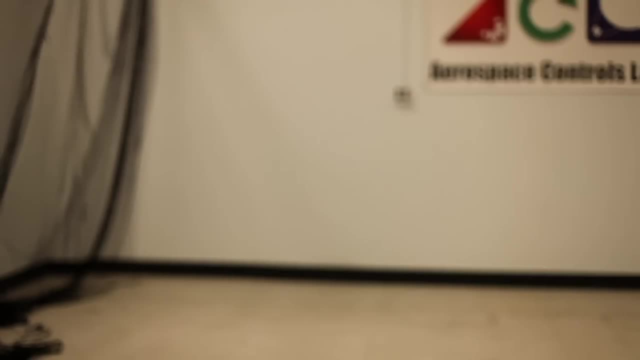 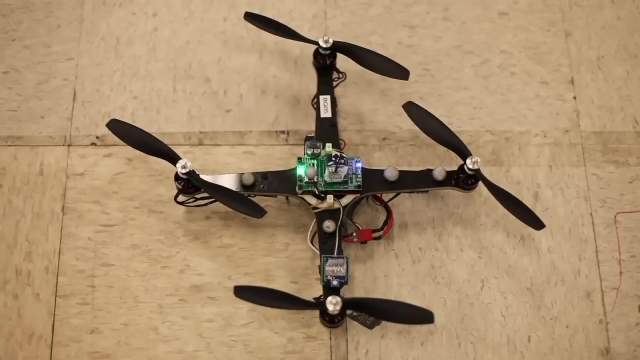 This introduces a horizontal force in addition to the one opposing gravity, and the vehicle moves sideways. That's great, but it doesn't tell us how the quadrotor can rotate about its vertical axis. It turns out that Newton's third law also applies to rotational force. 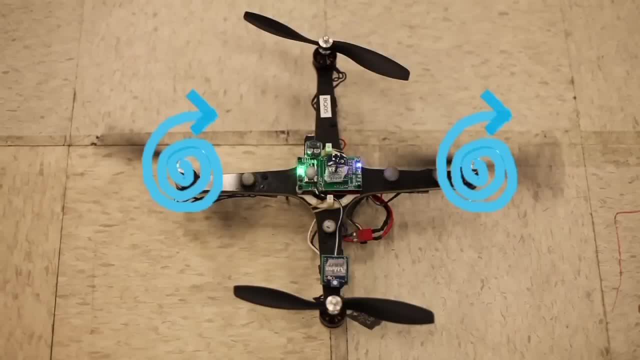 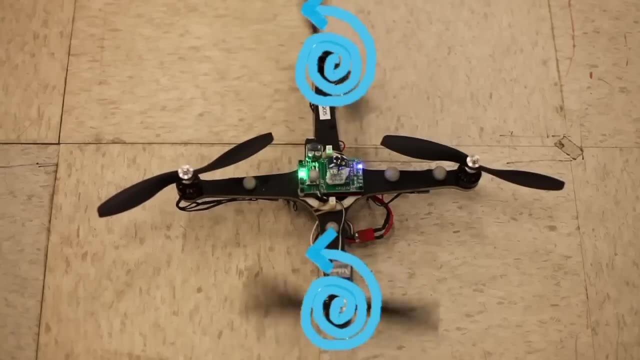 called torque. When these two propellers spin, they apply a torque to the air in the clockwise direction. The air applies an equal and opposite reaction torque, pushing the vehicle in a counterclockwise direction. Meanwhile the other two motors spin in the other direction. 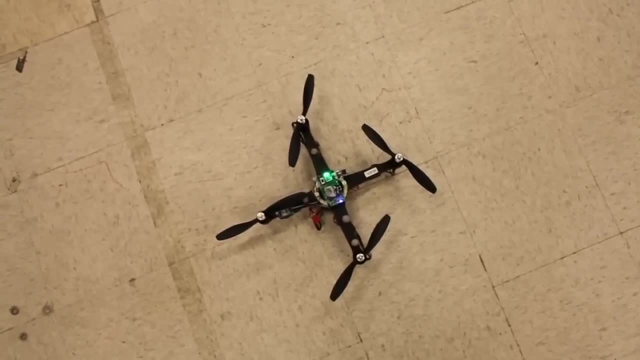 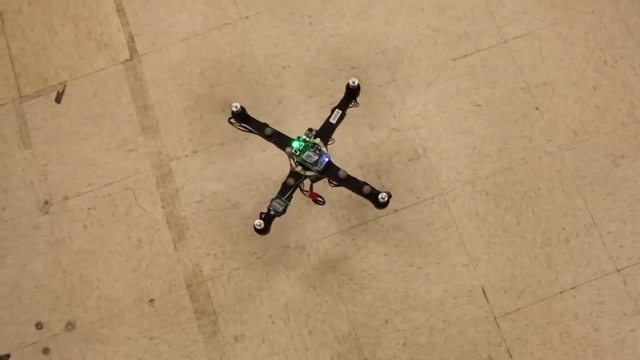 thus the reaction torque, pushes the vehicle clockwise. When all four motors are turned on, the rotational forces- remember they're called torques- balance each other In flight. the vehicle turns by spinning two motors ever so slightly faster than the other two. 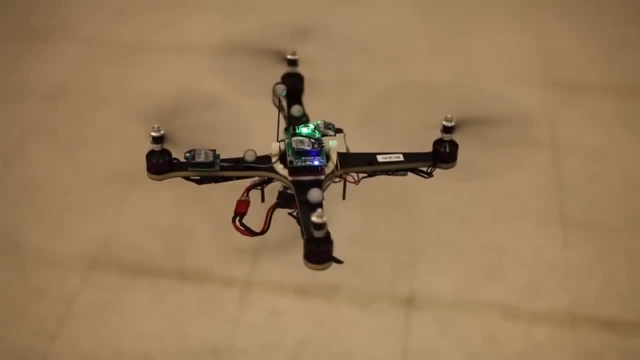 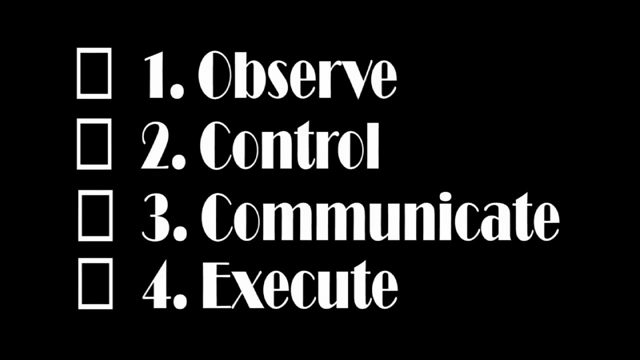 Now we know the basic physics of how a quadrotor flies, but before we can make it fly robotically, we need to know how to control it First. let's figure out how a human would do this. The task can be broken down into four key steps. First, the pilot uses his eyes to observe. 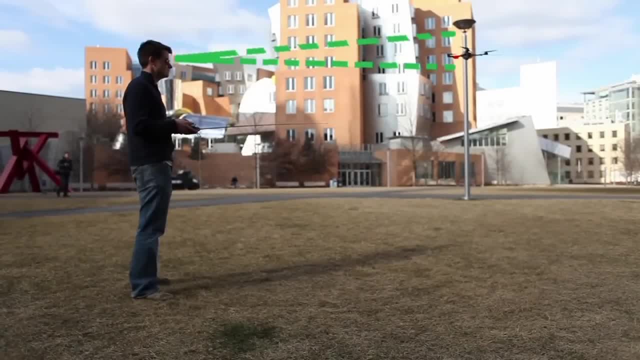 the vehicle and figure out where it is and in which direction it's pointing. In this example, let's say that the pilot sees that the quadrotor is moving in a counterclockwise direction and the quadrotor is sinking. Next the pilot has to decide what control. 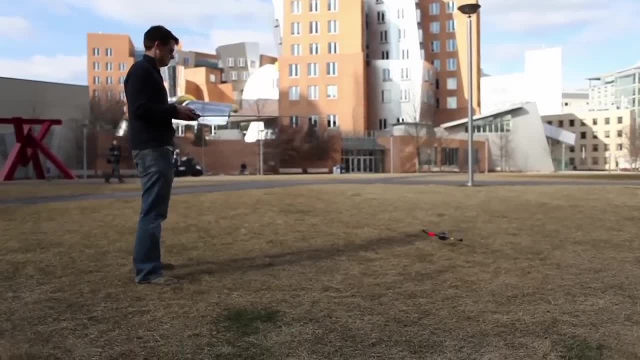 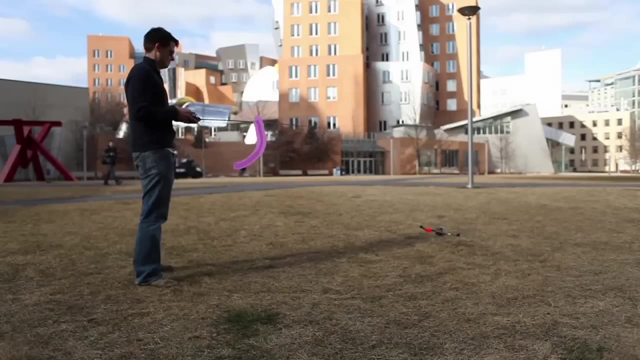 commands to give the vehicle. In this case, the pilot has to stop the vehicle from sinking, and thus decides to increase the speed of all four propellers. To tell the quadrotor what he's decided on, the pilot uses a radio transmitter, which is basically a fancy remote. 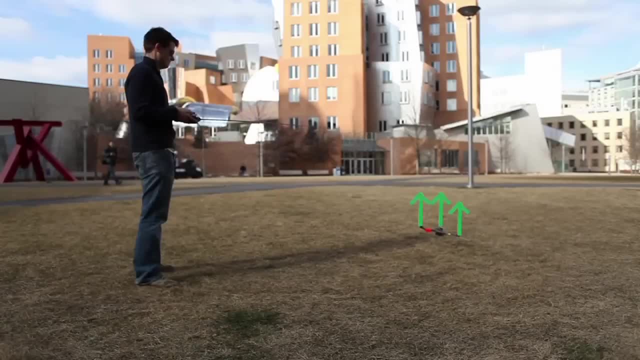 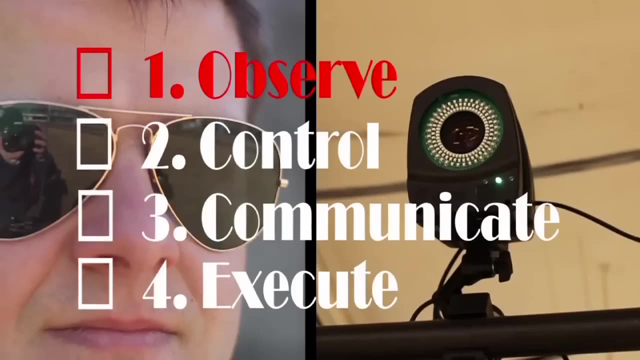 control. Finally, the quadrotor listens for the radio commands and adjusts the speed of each motor accordingly. Now let's see how each of these four steps changes. in order to make the quadrotor fly robotically In the first step, we use specialized cameras for vision instead of the pilot's eyes, The 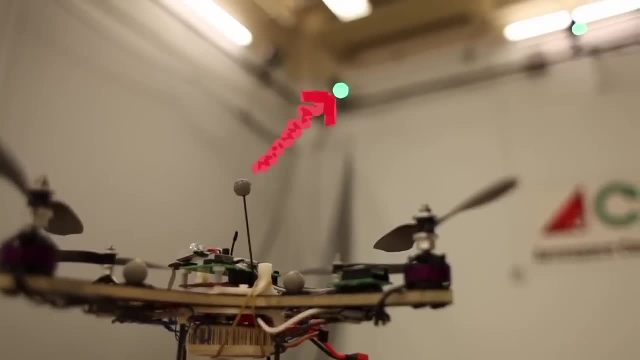 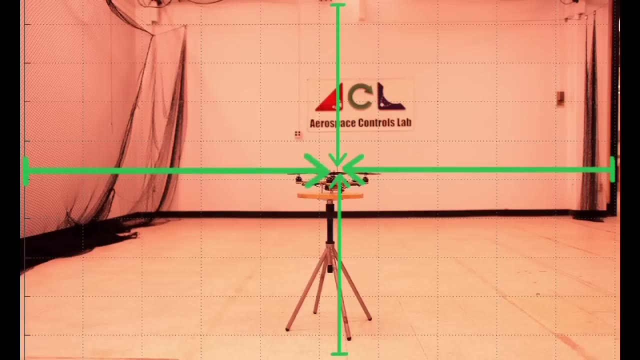 quadrotor uses infrared light which bounces off of small reflective markers on the vehicle and goes back to the camera. A camera from this side point of view can tell how far the marker is in the vertical direction and one horizontal direction, and a camera from this. 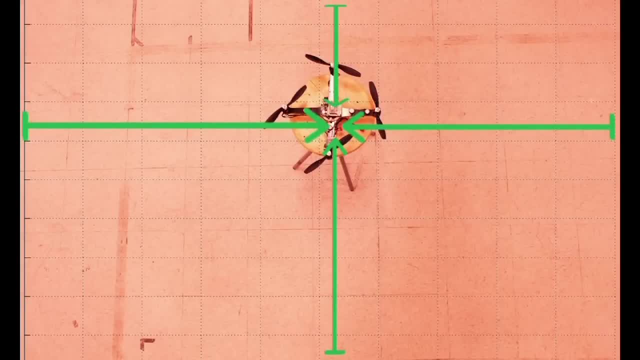 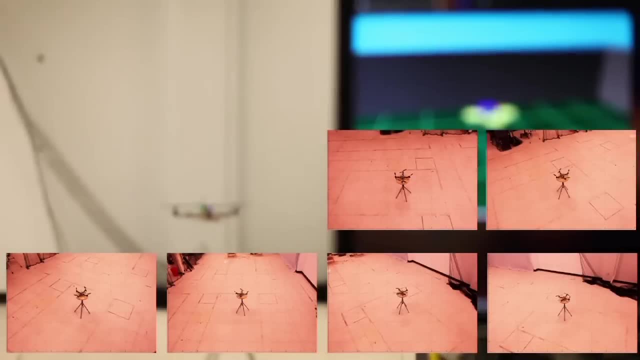 top point of view can tell how far the marker is in both horizontal directions. Using some slightly more complicated mathematics, we can use the points of view from twelve different cameras mounted along the ceiling to determine the exact three-dimensional position of the markers. This process is executed many times per second to track the position of 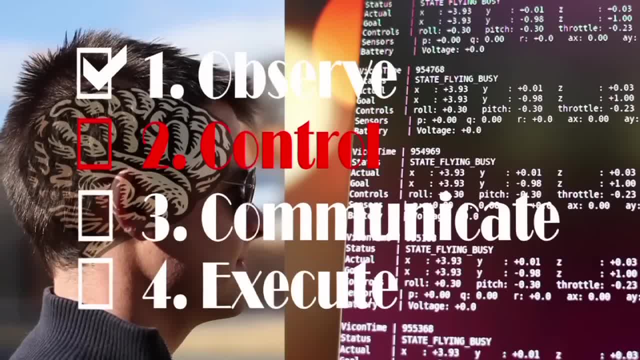 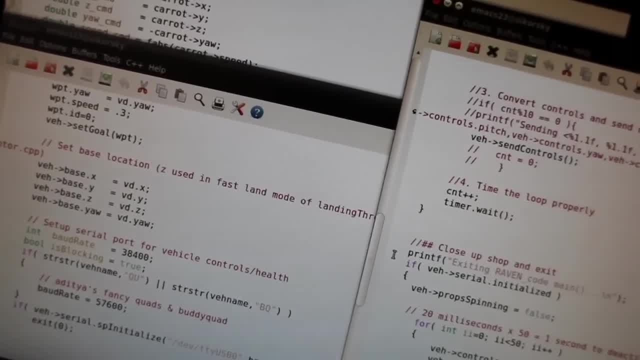 the markers, and thus the quadrotor, in real time. In step two, we use a computer to calculate the control commands instead of the pilot's brain. The computer program consists of a couple hundred lines of C++ code written by grad students who really don't get out much. It does essentially the same thing as 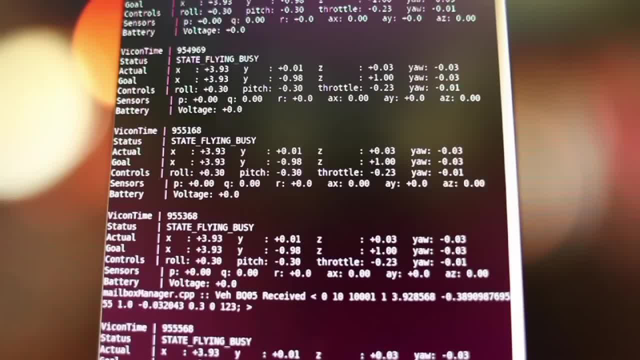 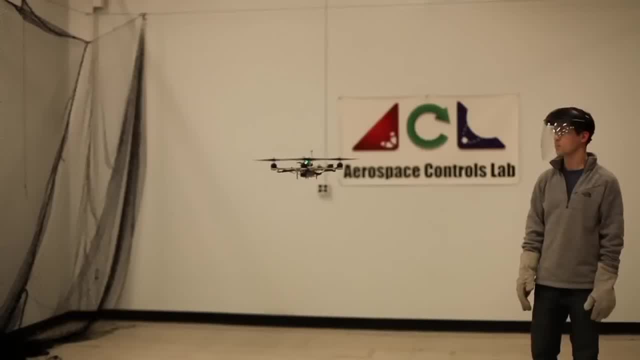 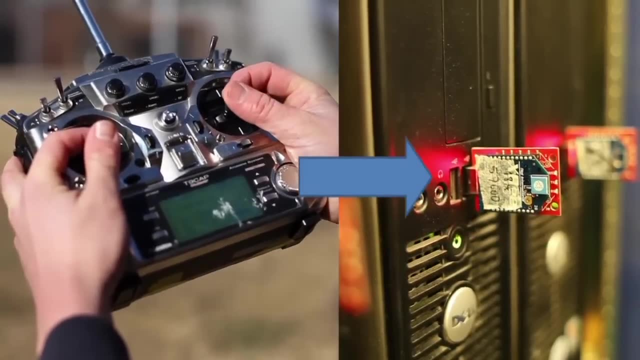 the pilot using the observed position of the quadrotor to calculate control commands, only it does so in a much faster and less dramatic fashion. In step three, the system uses a similar radio transmitter, except a smaller one with a lot of switches and control sticks. 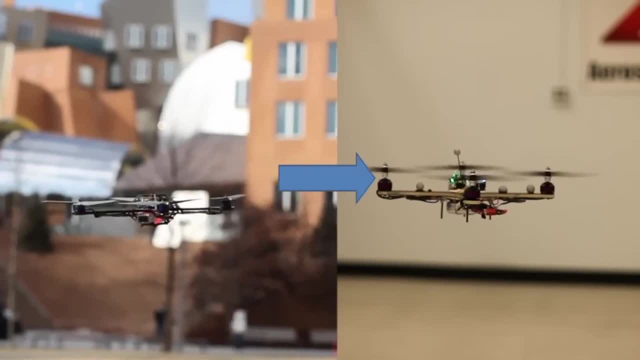 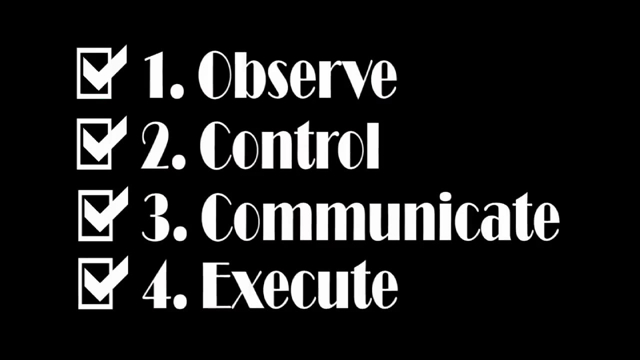 Step four is exactly the same as before. The quadrotor listens for radio commands and adjusts the speed of each motor accordingly. So we've updated all four steps in order to make the quadrotor fly entirely by itself. Now all we need is for our grad student to press the. 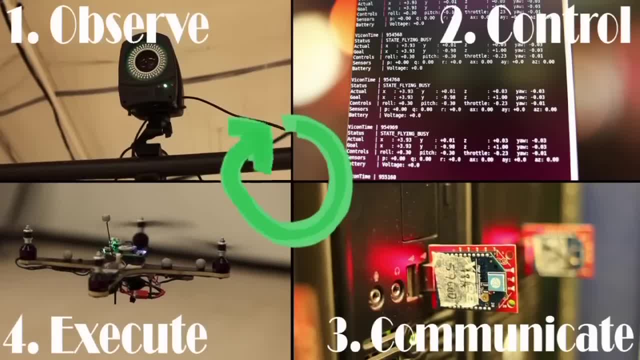 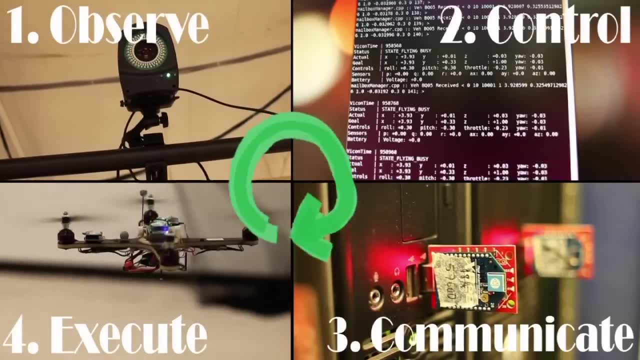 go button and voila. One of the reasons the robots fly more precisely than the human pilot is because this loop of information, called a feedback control loop, can be executed much more quickly by computers, in this case, two hundred times per second. 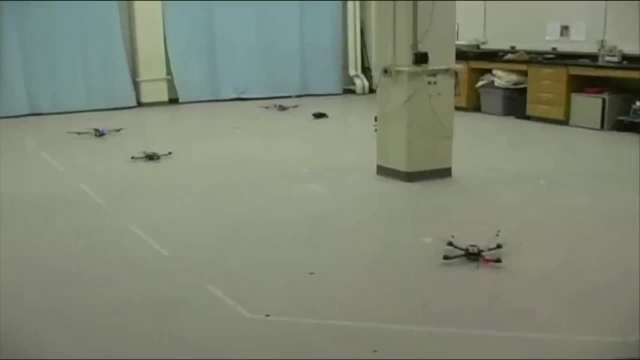 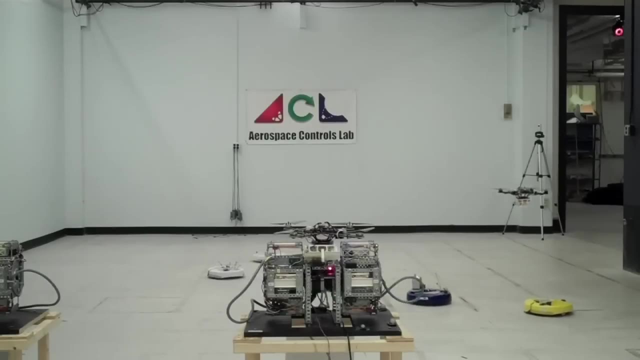 This allows researchers to do cool things with these indoor flying robots. For instance, fly six of them at once, Or why not ten? They can teach the vehicles how to switch out their old batteries for new ones automatically or stop a payload from swinging. They can. 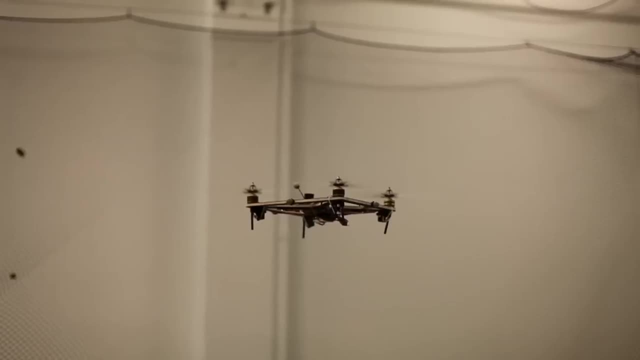 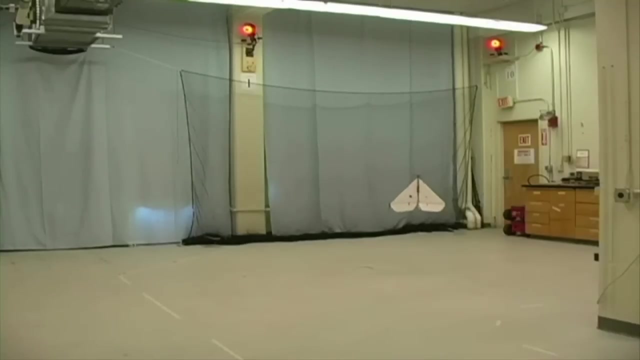 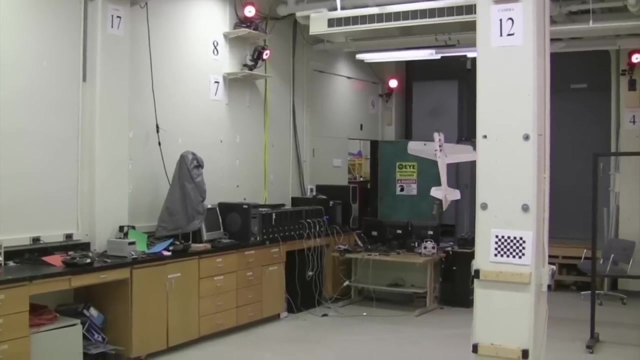 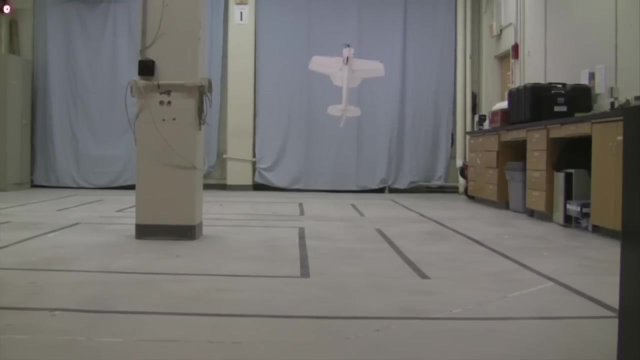 even do flips like this one, or this one or this one. And the fun doesn't stop with quadrotors. The same technology can be applied to weirdly shaped quadrotors, Or three wing of madoobers, Or more conventional fixed wing vehicles like this one, this one. 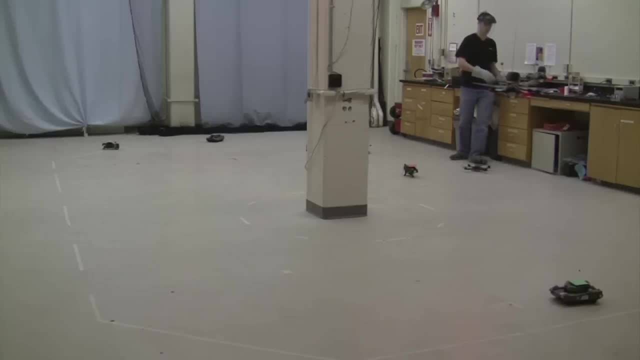 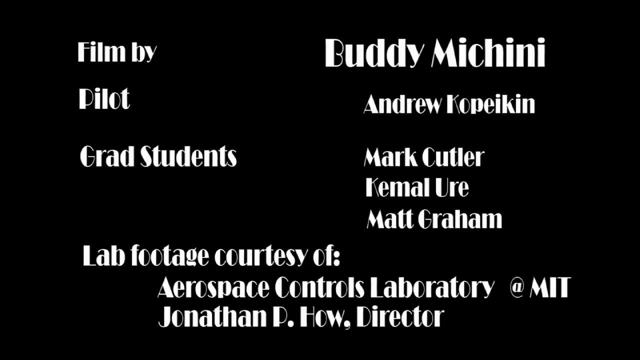 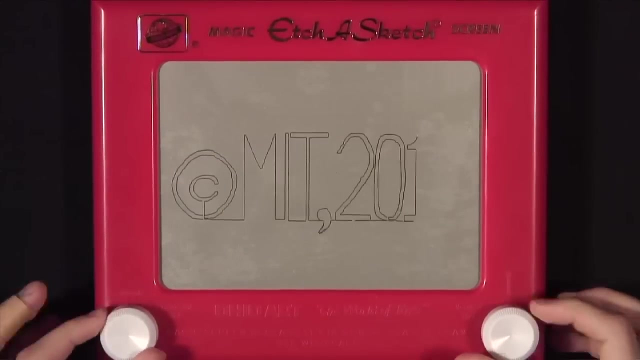 and this one that can even fly loops. Well, hopefully you've learned the basics of how to make robots fly. This concludes the crash course. I mean expedited learning experience. See you next time.